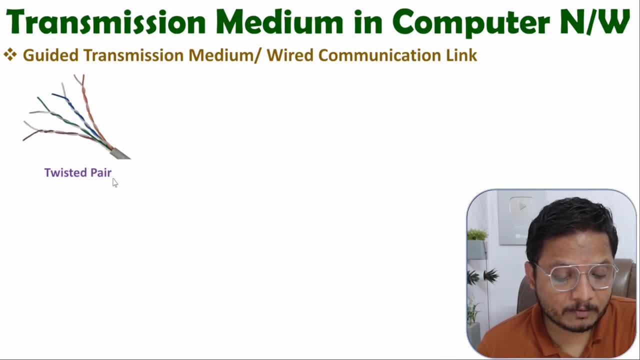 So that is there as per twisted pair. First you need to see this diagram. You see we are having one cable over here and inside this cable how many twisted pairs are there? You see, this is one twisted pair, This is second twisted pair, This is third twisted pair and this is four twisted pair. So with this given cable, we are having in total four twisted pair Right now here in twisted. 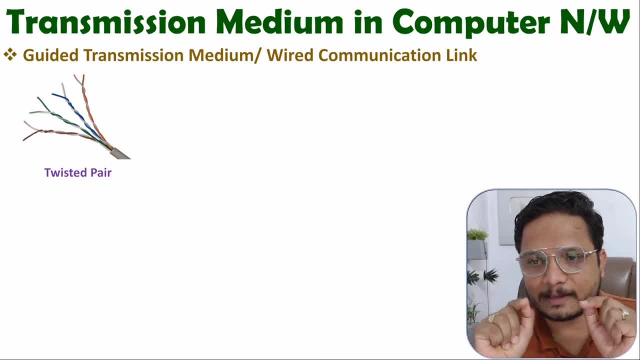 pair. what we do is we insert electrical signals Right, So with one twisted pair we can provide electrical signaling. Likewise, here, with this particular example, we are having four twisted pair Right Now. let me tell you the brief history about this. Like this twisted pair cable that we were been using in early 1990s with telephone network- See, in 1990s telephone network was providing 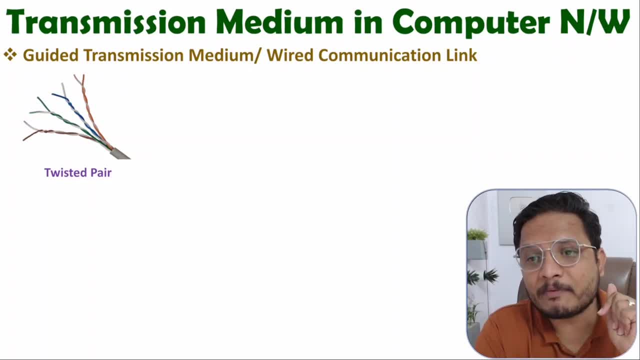 internet connection Right In that, this type of cable that we were been using in that 1990s period. Right now probably you can observe we are using ethernet cable, optical cable, Right For internet connection. But in early 1990s internet was deployed along with telephone line, where this type of cable was there. Right Now, here see, it is a pair of two wires that you can say with twisted pair and earlier telephone network. 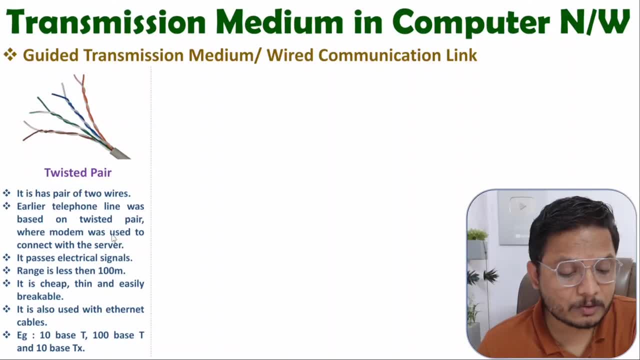 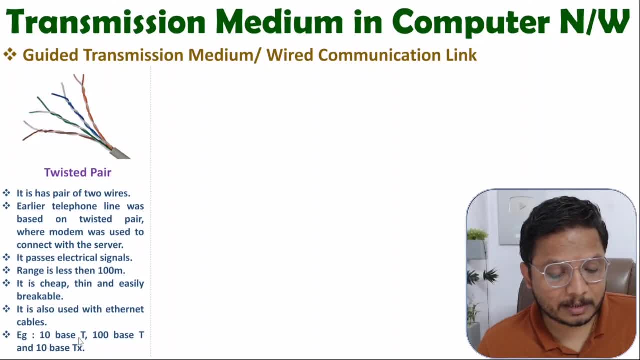 cable And you see here few examples are given for ethernet cable And I have seen some questions are frequently coming based on what type of ethernet cable that is given, based on some notation. So here if I say tan, base T, that cable is given to you, then what is the meaning of this? See this: tan means tan mbps. speed is there with this given cable and base T means here with this given table cable, we are having one. 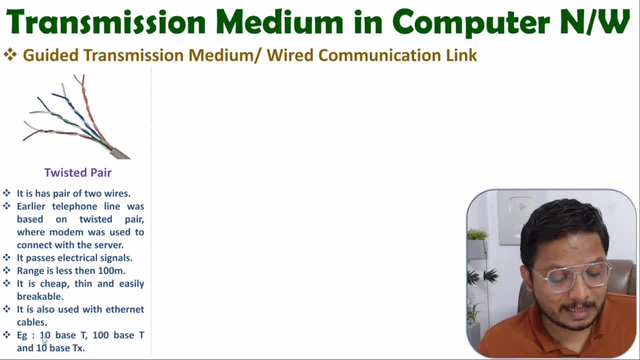 twisted pair. So tan base T means tan mbps speed is there with the cable and T means only one twisted pair is there. So with this cable we are having four twisted pair, But with tan base T cable you will be having one twisted pair and speed will be tan mbps. When it comes to 100 base T type of twisted pair cable, in that case you can say speed is 100 mbps and base T means what T indicates there will be. 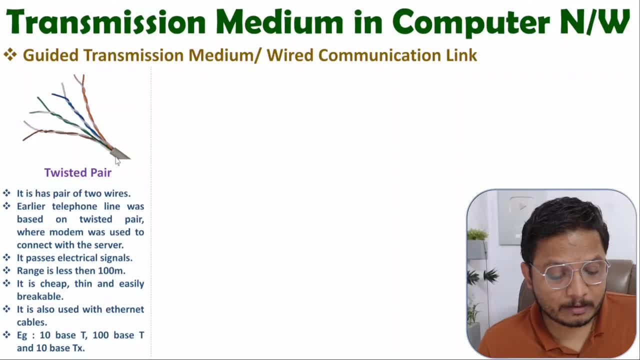 only one twisted pair inside given cable. When it comes to 10 base TX, what it means? it is 10 mbps and TX means there will be two pair of twisted pair cable, Right? So inside cable there will be two pair of twisted pair. So here, one and two. That is how two pair will be there here. in total, four pairs are there, Right? So, as if you wanted to know, like, what should be the notation for four pairs. 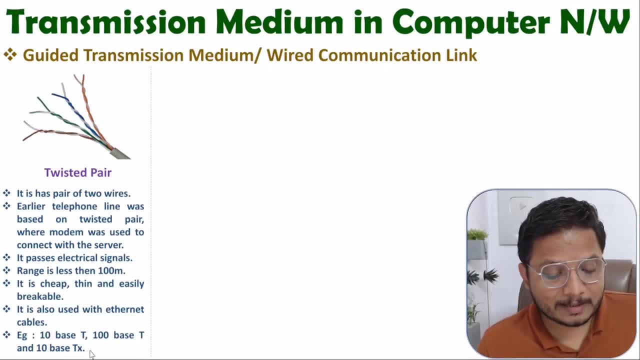 four twisted pair cable. so for that i can say tan base t4. that will be written. so tan base t4 means what tan will be, the tan mbps will be the speed and t4 indicates there will be four twisted pair. so based on notation, you should know what kind of cable is given to you. so this type of questions. 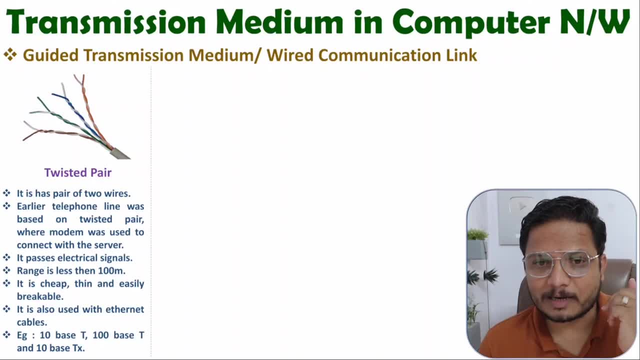 that may come in competitive examination. right, it is quite easy. i think you can easily understand that based on these examples. now let me explain you. second type of guided transmission medium where you see shielded twisted pair that we have. so here we are providing shielding of copper with. 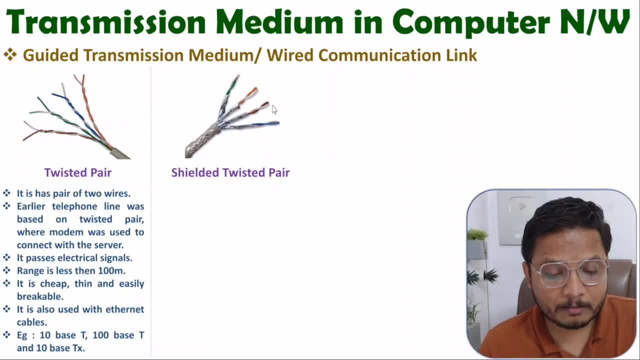 twisted pair. you see, here we are having four twisted pair, but all the twisted pairs are provided with aluminum foil shielding, right? so you see, entire cable is getting shielded over. here and here aluminum foil shielding is happening. you so, this and this cable. both are similar. only difference is shielding is there. now what will? 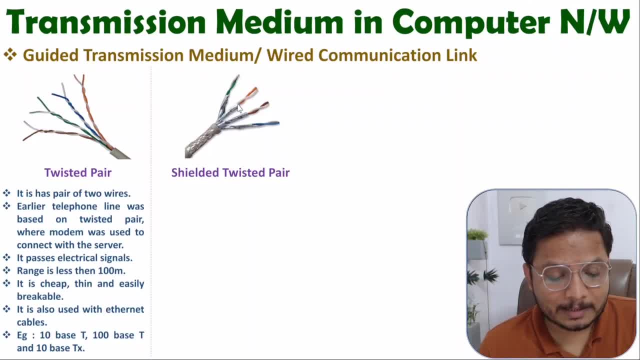 happen because of shielding. see, one thing that will happen is, like you can say, this cable that will be stronger than this cable that you can directly say. and secondly, because of shielding of aluminum foil over here, there will be less interference of signal in between these two cable. 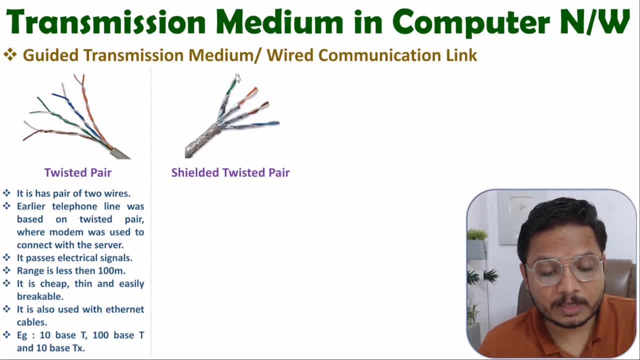 right, like in single cable, there are how many twisted pair? you see four twisted pairs are there. so if you provide aluminum foil shielding over here, then noise will reduce in between this cables which are there in this twisted pairs which are there inside this cable, right? so that is the basic logic behind this. 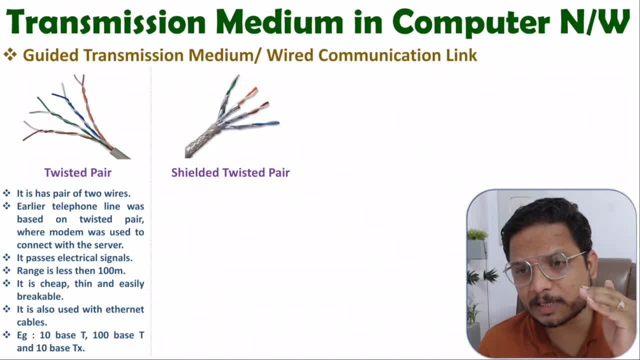 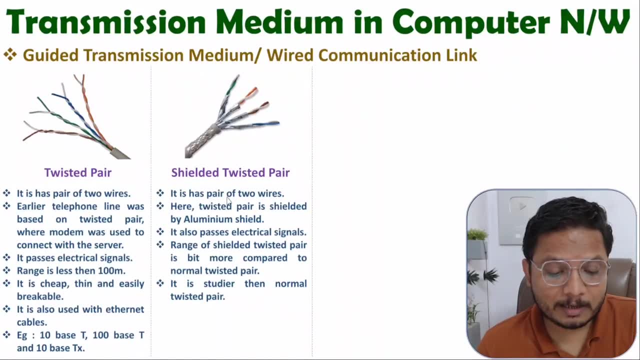 like, by providing aluminum foil shielding, we are reducing noise as well as we are increasing the strain. so you see, here we are having two pairs of wires. only thing is we are providing aluminum shield over here, so individual shielding is happening as well as total wire shielding. that is also done over here, so it is increasing strength and it is reducing noise. 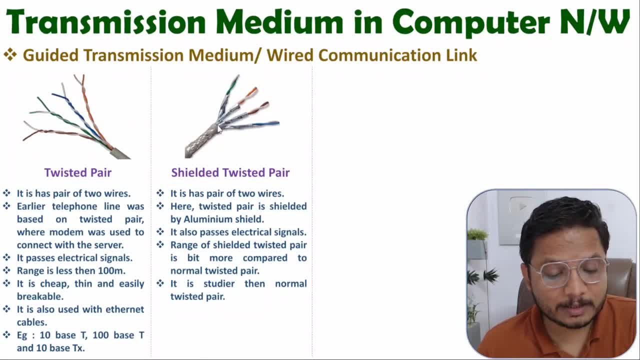 inside propagation of signal and because of reduction in noise range will increase. so range of this tilted pair with twisted pair you can say it will be bit more compared to this, so you can say it is steadier than the normal twisted pair. why the reason is: here we are providing aluminum. 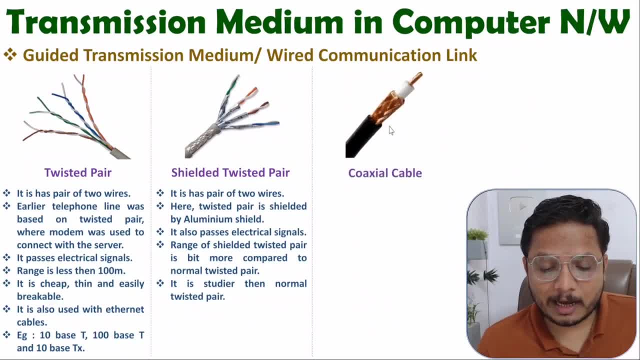 shield. right Now let us try to understand how hard guided transmission medium cable is. there like coaxial cable, and I think you might have seen that in your television connection, right? So for television connection we use this coaxial cable. If you open up this coaxial cable, it will be looking like this, where this is inner conductor and outer conductor is separated by dielectric material and this is a cover of that entire cable, right? 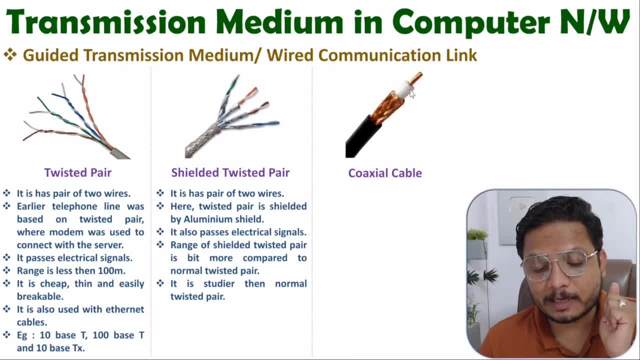 So here what will happen is you see signal that will be passed on with respect to these two wires, only right, And I have seen students are thinking like: here also we will be sending electrical signals, only right. So you can say it could be electrical signal, but not exactly the electrical signal which will be available over here right Here. signaling will be very different with this coaxial cable. 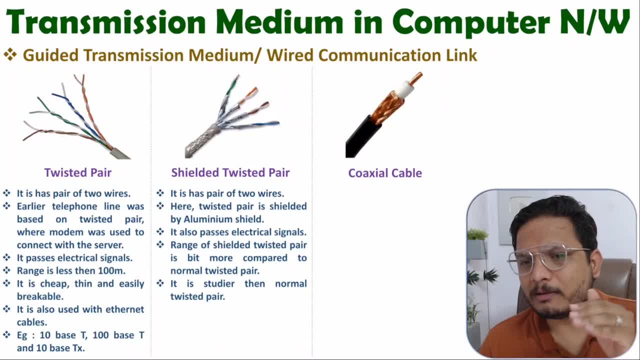 When we talk about coaxial cable, you should know, even this coaxial cable, that we use it in television connection means with our TV. we are having this, as well as with some broadband, broadband services. we are having this type of cable and right now also with large scale, this coaxial cable that has been used right In 2023, this coaxial cable that has been implemented in many computer network. Now let me tell you some basics about this. 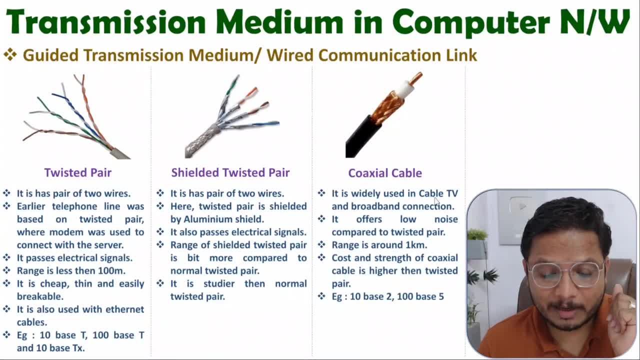 Like you see, it is widely used in television of cable television and in broadband connection that we use right. It offers low noise compared to this twisted pair. That's why its range is more. It is there in terms of one kilometer right And cost and strength of this coaxial cable. that is a bit more compared to twisted pair cable. 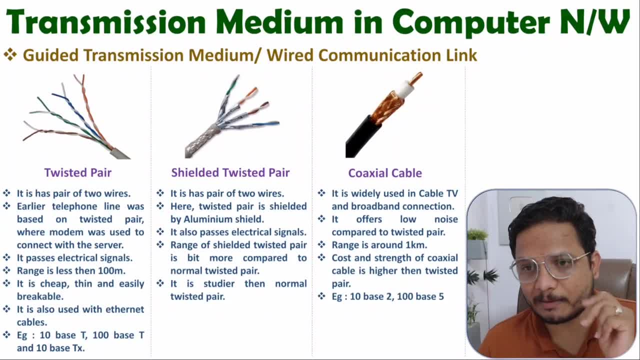 Now I have seen some questions are coming based on notation of cable, like as if it is given there is two kind of cable is given to you, Then you should know this cable category that comes under the category of coaxial cable first, and there's two. means what? and is a speed in terms of MBPS and base. two means what? two into hundred meter distance means two hundred meter distance that is been supported by this given cable. So for two hundred meter distance we can use that cable right. 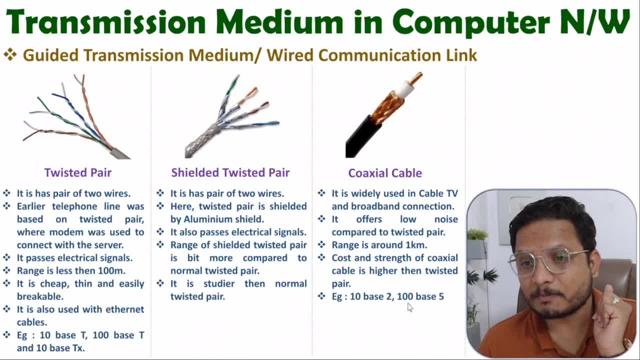 Base five means what hundred is MBPS speed, which is there with given cable, and base five means five into hundred, means five hundred meter distance communication. that is possible by this cable right? You see, here with twisted pair it will be given in terms of 10 base T, So here T indicates how many pairs are there, while with coaxial cable it will be given in terms of this like 10 base two, So here two gives you the distance of communication. 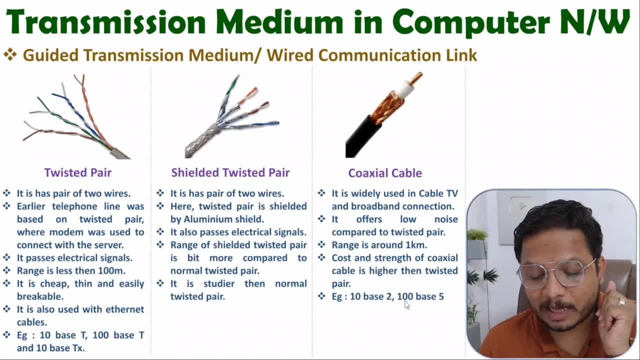 With this given cable two into hundred, right, Like sometimes they may give you, like this, hundred base six. So hundred is MBPS speed and six means six into hundred, means six hundred meter distance, that will be there with that cable right. Now I'm going to explain you third category of cable, that is optical fiber, right? So in this you see we are having optical fiber. 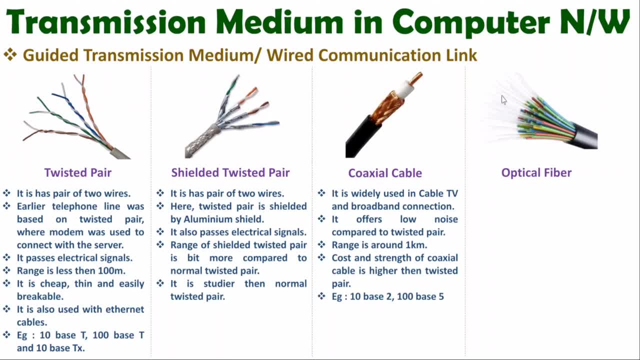 We are having optical fiber cable where signaling will happen in terms of light signal and for wide band application we use optical fiber. that you should right. Right now current internet connection with computer network that is having majority of base with this optical fiber connection only right, If you see the basics then you should know it is working based on light signal. It is having very low noise interference compared to optical fiber. 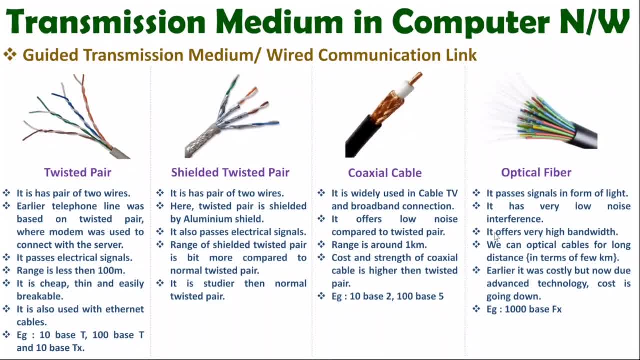 All these cables. that's why it offers very high bandwidth as well, as we can use this cable for long distance. Why The reason is it is having very low noise interference. inside and in single cable you can observe how many fibers are there. You see, with this coaxial cable we can have signaling with one line only, right, But over here, with this optical fiber, you see how many fibers are there inside, So that many fibers are there inside. 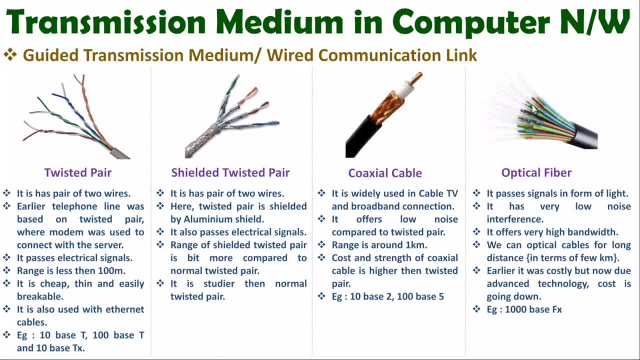 You can have individual, separate bandwidth, right. So in short, you can say: with single fiber cable we can have many microfibers inside and that leads to huge bandwidth. Each fiber inside single link will be having bandwidth in terms of 100 Mbps, So as if you have 10 fibers inside a single cable, then you can say: 100 into 10 means you can have 1 Gbps speed, right, So it offers high bandwidth. 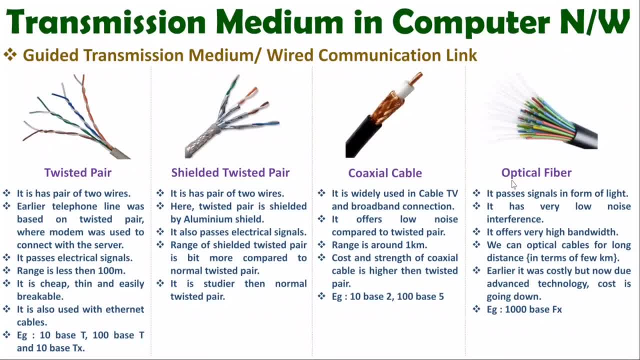 Very high bandwidth. That's why, in majority of computer network you will be observing optical fibers are connected. right, You can say it is costlier earlier, but because of some advanced fabrication technology, nowadays, in 2023, cost of this optical fiber, that is going down Now. here also one example is given, like if cable is given as per this 1000 base FX, what it means 1000 is. 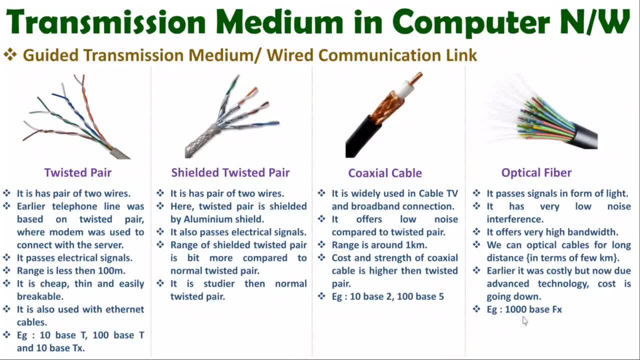 a speed means 1000 Mbps. speed is there with given cable and FX is optical fiber extension And with this FX notation you can say distance of communication will be 2 kilometer approximately. So this cable that could be used up to 2 kilometers, right. Likewise, as if it is given like 100 base FX, then you can say 100 will be, 100 Mbps will be the speed and FX explains you: optical fiber cable is there. 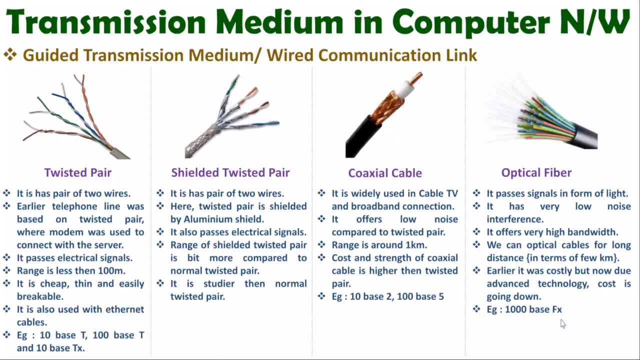 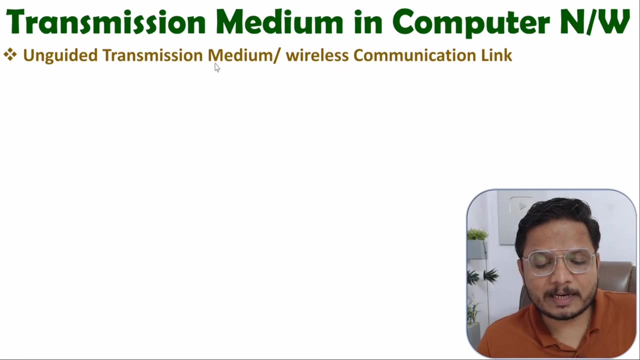 And with FX standard notation is there as per 2 kilometer distance, right. So that is how notations are there with different cables. So you should know about this basics of notation with cables right Now I'm going to explain you. second category, that is unguided medium. So in unguided medium we can say it is wireless communication link And in that there are two categories only. 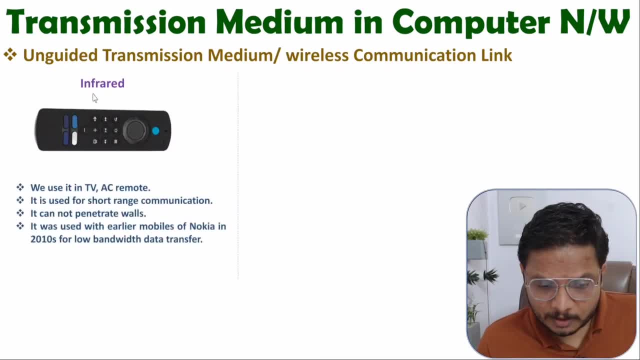 One is infrared and second is radio wave. In infrared you will be observing, We use that for short range communication and many applications that you might have seen, like TV remote control or AC remote control. So in that we will be using this infrared medium right, It cannot penetrate through wall right. So that is the biggest disadvantage of this infrared communication link And you will be observing in unguided medium. 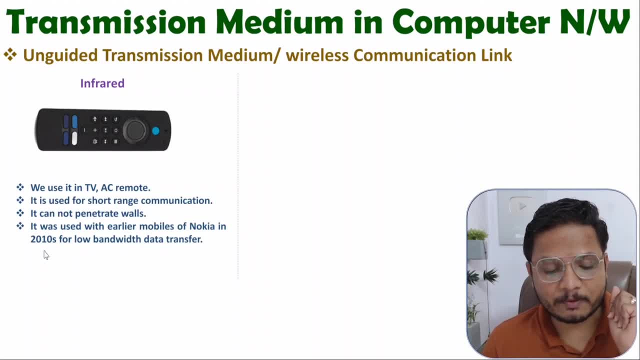 Earlier mobiles of Nokia in 2010s, we were been having low bandwidth data transfer as per infrared wireless link. So I was been using Nokia's N73 mobile in that infrared data transfer technology was there right. But because of there are many disadvantages with this technology, majority of applications were not utilizing this. Right now, infrared communication that is there with the application which is there, based on remote communication. 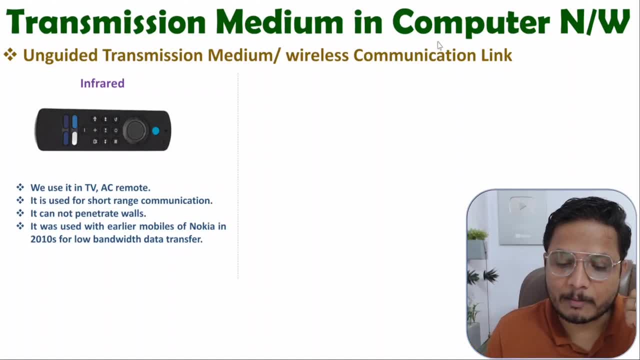 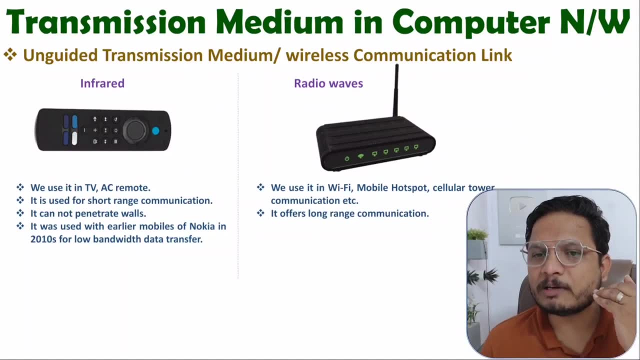 But because of the huge frequency of ARP also, it is difficult for us to bring like WiFi where we can walk around in front of it and use the remote control only right. So environment network: we will be observing. usually We use radio waves and this radio waves that we use it with WI-FI, that we use it with cellular tower, as well as with your mobile phone, called sport, We can use radio.